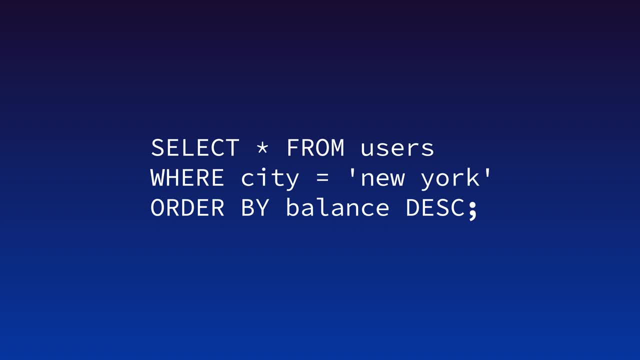 life. often we might not really need the information from each column. Imagine, for example, that we just wanted to get the IDs for each New York user sorted by their account balance. When we explain, analyze this query, we can see that we're down to a single column. In the example query, we can see that we're down to a single column. Imagine, for example, that we just wanted to get the IDs for each New York user sorted by their account balance. When we explain, analyze this query, we can see that we're down to a single column. In the example query, we can see that we're down to a single column. When we explain, analyze this query, we can see that we're down to a single column. And this is a soupy little step thanks to our index and the fact that we're now pulling. 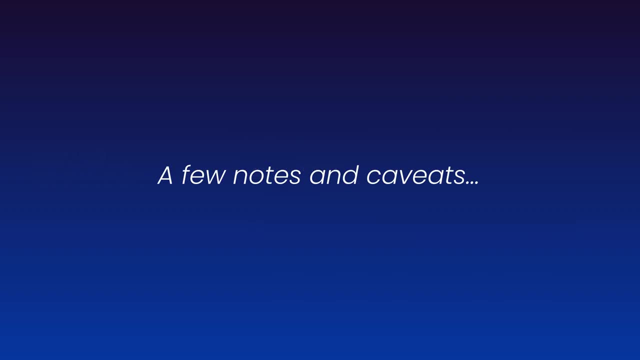 only the data that we actually need. Obviously, we can't create unique indexes to optimize for every possible query that might be run against our database, And there are some important caveats here. Number one: indexes do have to be kept updated, which means that write operations have to. 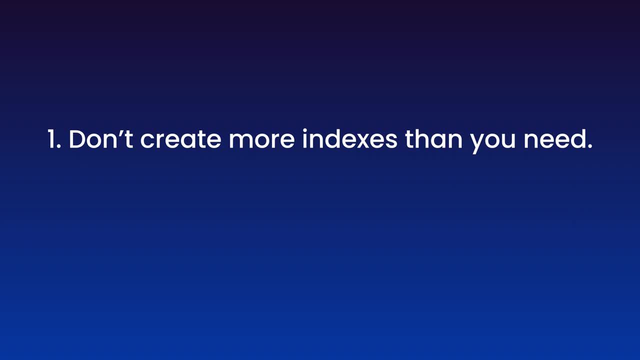 write to any index that's impacted as well as writing to the table. If you build too many indexes and each write has to update them all in addition to the table itself, that can slow down writes. so in general, don't build too much write in in the index. 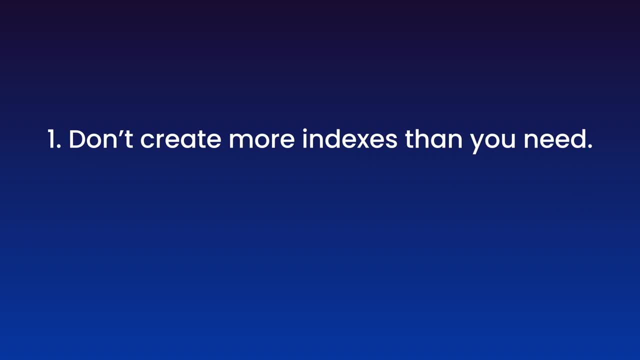 many indexes stick to just what you need to optimize for the most common types of queries. Second, indexing on a large field will result in a larger index. For example, indexing an emails table on its body column, which might contain paragraphs of text for each row. 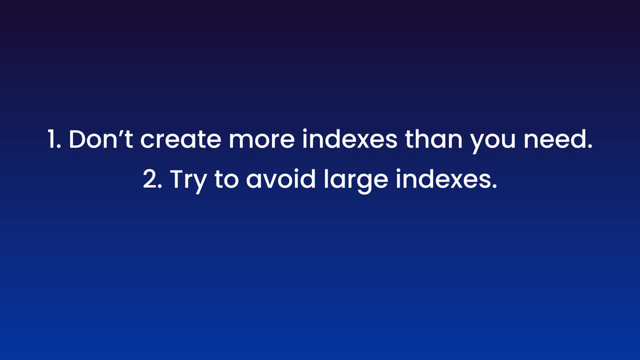 will result in a larger index than indexing on a smaller column, such as date time, which will contain fewer total characters. Where possible, avoid indexing large fields. Third, when in doubt, explain What we've talked about in this video provides a good 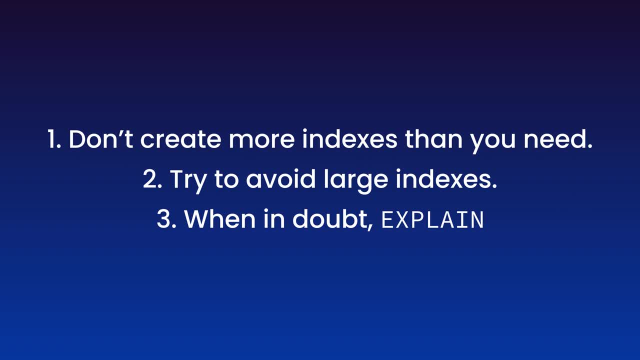 general guide to optimizing your SQL queries with indexes in CockroachDB and in most other SQL databases, But no single approach is going to be best for 100% of use cases. Remember that you can always use explainanalyze to check out how a query will be executed and. 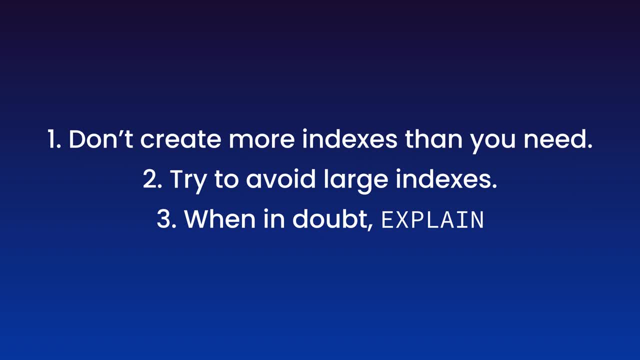 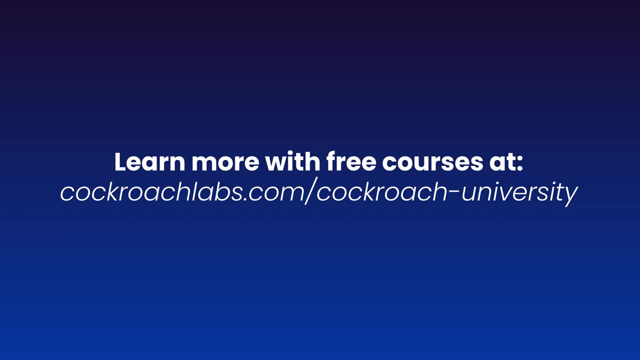 to test different approaches to see which one is the most efficient. Still have questions? We've also got a blog post on this topic, linked in the video description, Or you can check out Cockroach University, our free online learning platform with interactive courses specifically for you. 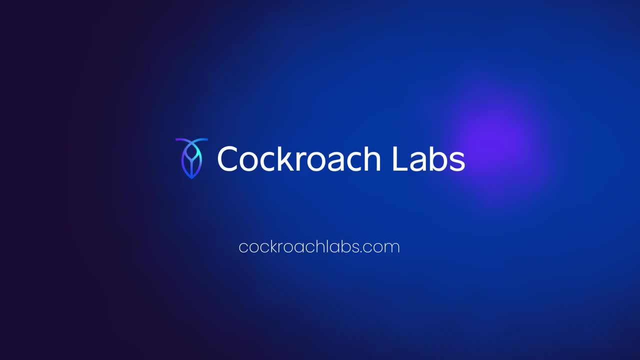 It's perfectly designed to help you get the most out of your SQL database.